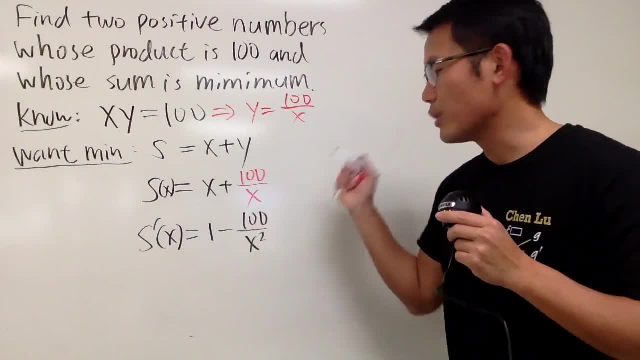 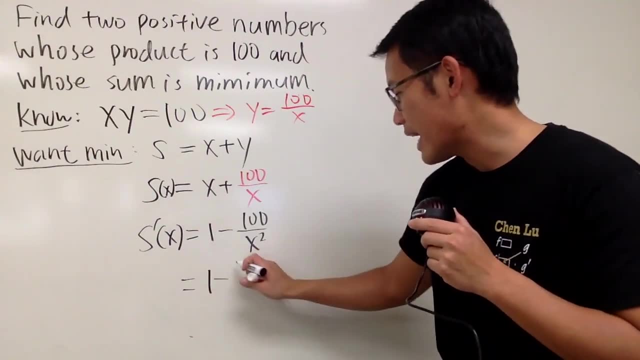 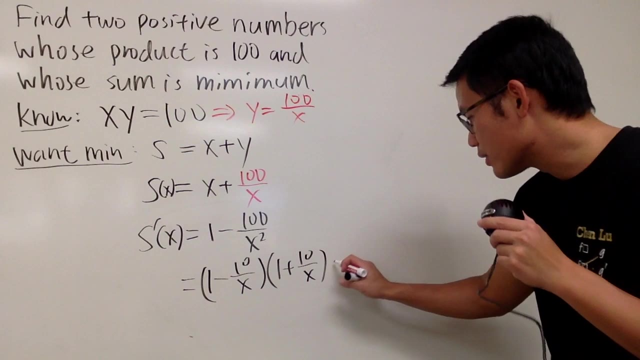 Don't forget the 100 on the top. so we have 100 over x squared like this And in fact- let me factor this a little bit- This is the difference of two squares. so I will go ahead and do 1 minus 10 over x times 1 plus 10 over x, And, as usual, let's go ahead and 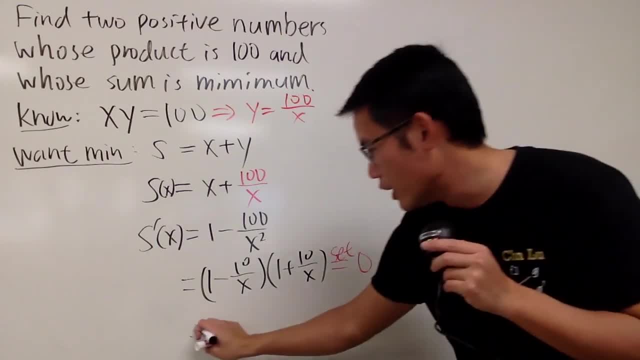 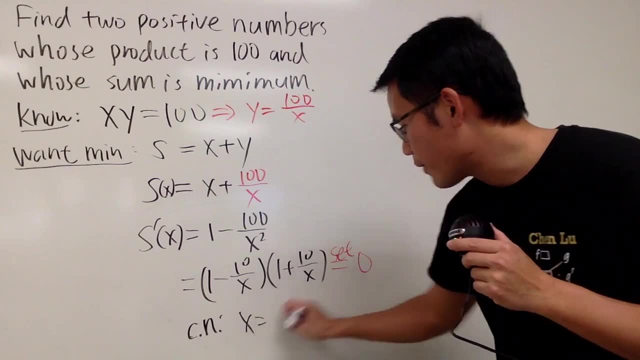 set this to be 0, so we can find out our critical numbers From here, as we can see, we need x to be 10, and from here we can see that we need x to be negative 10.. And in fact we don't. 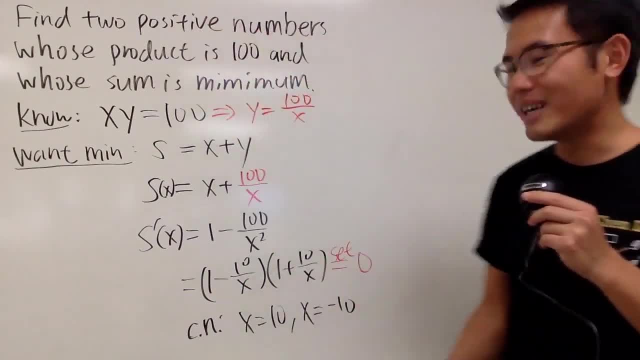 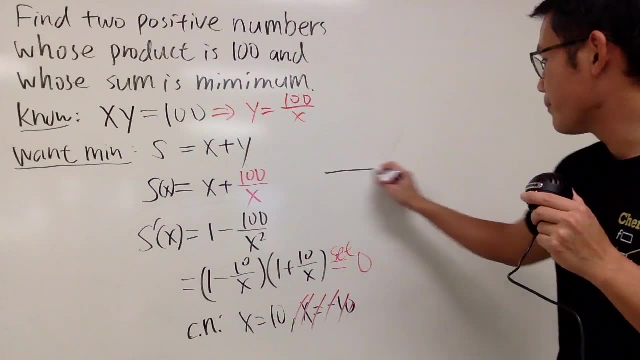 need to care about negative 10, because we're looking for two positive numbers, right. So this right here is actually out of our consideration. And now let's just do a number line test real quick. so I will just put this down right here: This is x and this is s prime. so which? 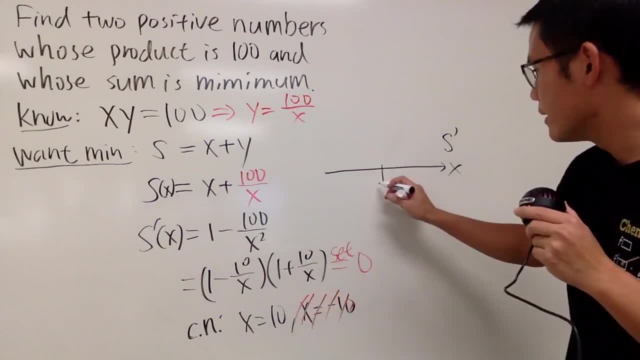 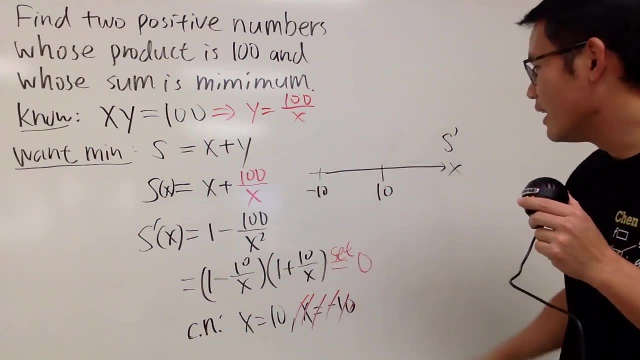 is the first derivative. Okay, so now we have our negative 10 over x, so we can find out our critical numbers over to right here. just focus on 10. right, and technically negative 10 is right here, but again, maybe i'll put it down just to not let it feel left out. anyway, i have to pick a number. 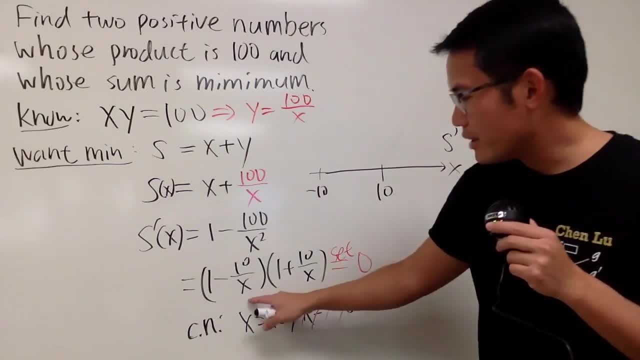 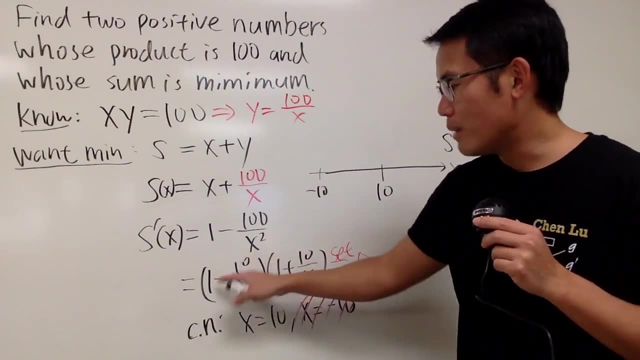 slightly less than 10, let's say 9, put the 9 right here and right here. when we do 9 here, this is 1 minus 10 over 9, which is bigger than 1. 1 minus something bigger than 1. we get negative, and then 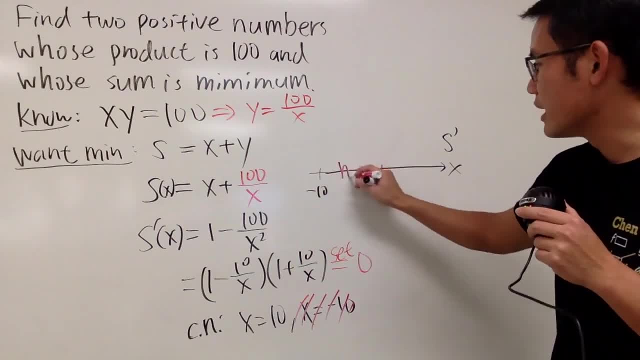 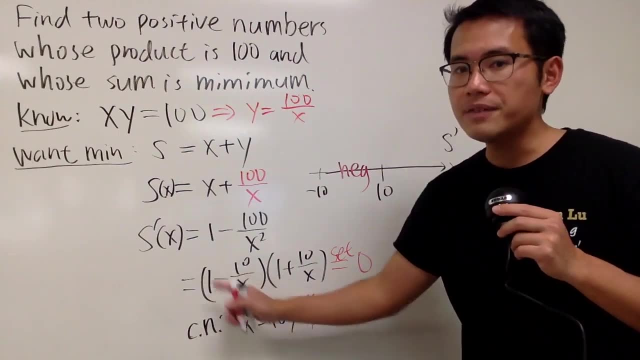 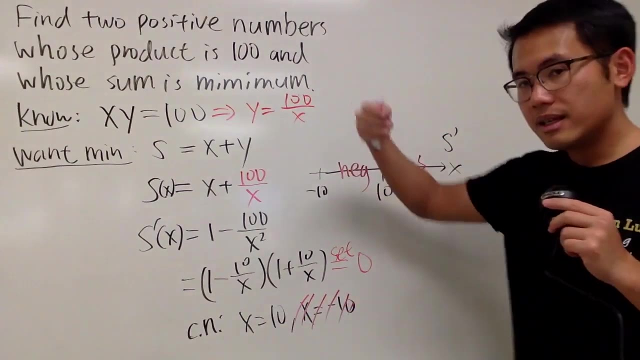 that will give us positive. so, in fact, this portion here is negative. and when we have a number bigger than 10, let's say 25 or something, that would be positive, that would be positive, so we have positive. so, as you can see, when x is equal to 10, we actually get, you know, the function going down. 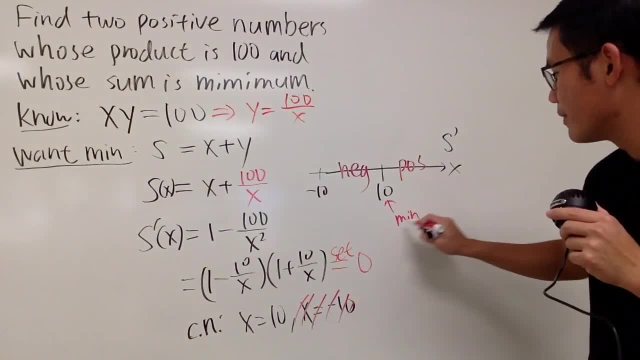 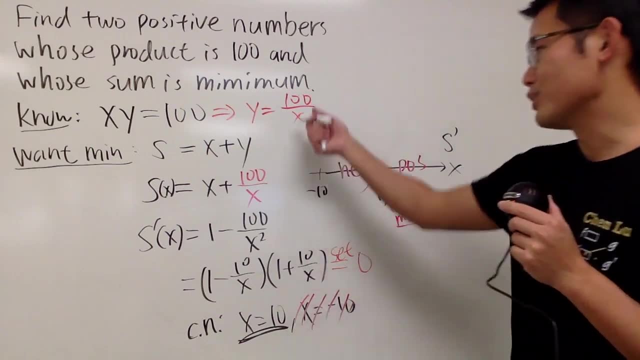 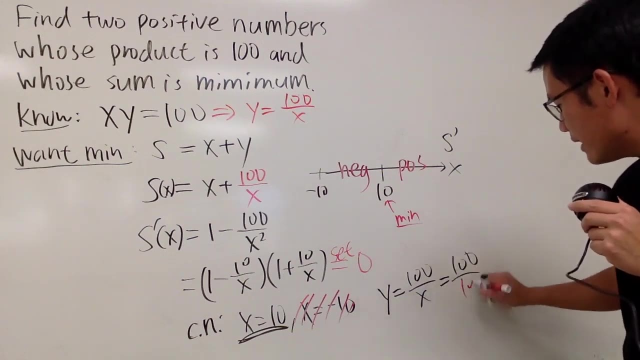 and then go up. therefore, this is a minimum right. so this right here is what we are looking for. x has to be 10. how can we find y, though? just go back here. so, of course, y equals 100 over x, and that's 100 over 10, which is, of course, 10. 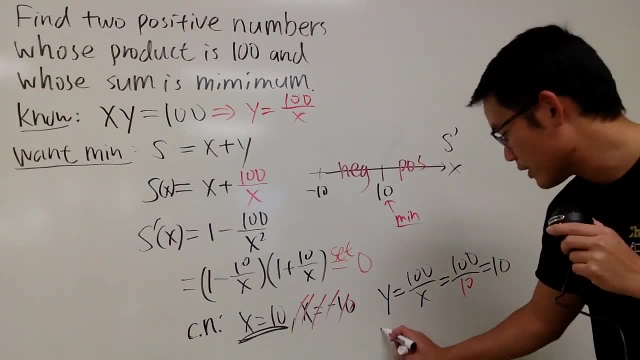 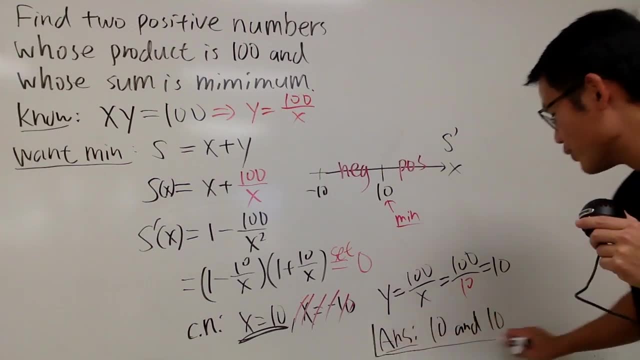 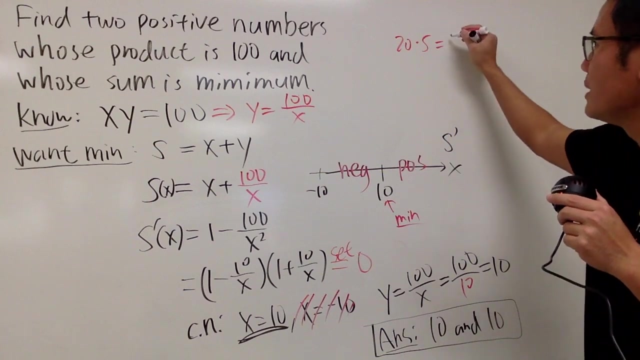 so i will just tell you guys right here, right? so the answer is just going to be 10 and 10 and of course, when you multiply 10 and 10, you get 100. when you add them up, you get 20 and if you look at, let's say, 20 times 5, this is going to be 100 as well. but if you do 20 plus 5,